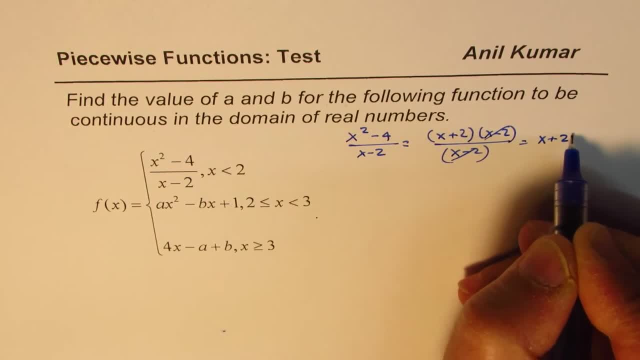 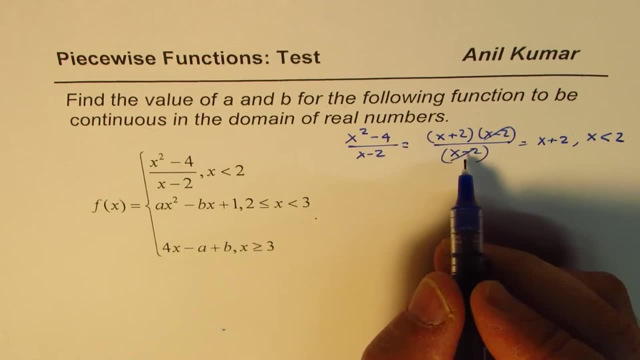 over x minus 2.. This cancels out, So we get x plus 2.. Remember, here, since x is less than 2, we could cancel this out. right? We know x is not equal to 2.. OK, So that's fine. So this function. 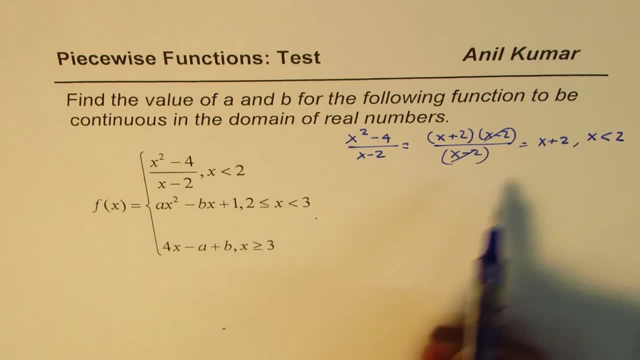 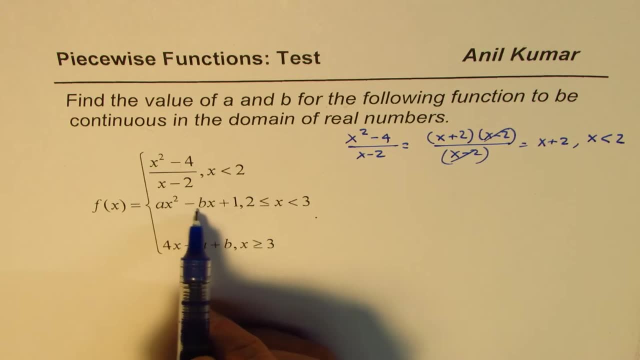 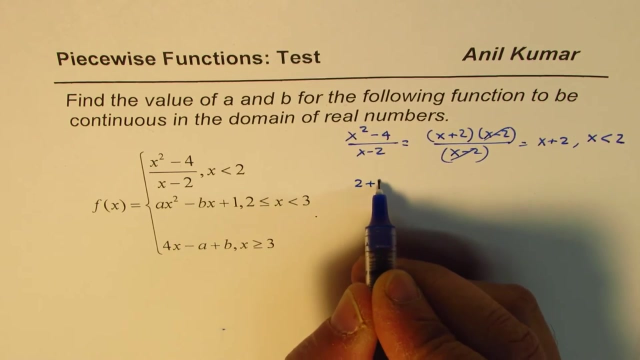 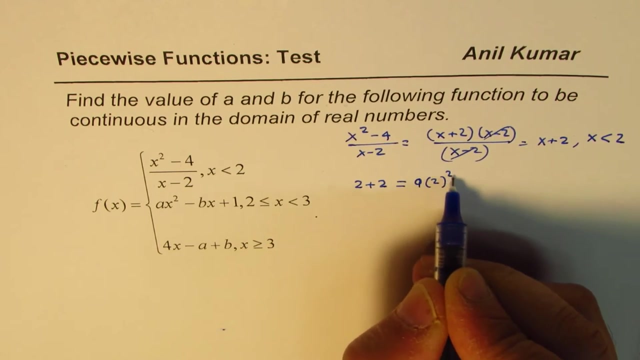 could be actually written as x plus 2.. Now the idea is, what is the value of this function at 2?? It should be seen as the value of ax squared minus bx plus 1 at 2, right, So we can substitute 2 here. right, So we get 2 plus 2 should be equals to substituting 2 here. we get a times 2 squared. let me write this: minus b times 2 plus 1.. 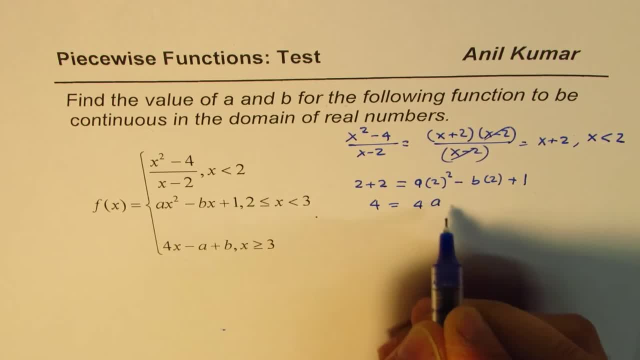 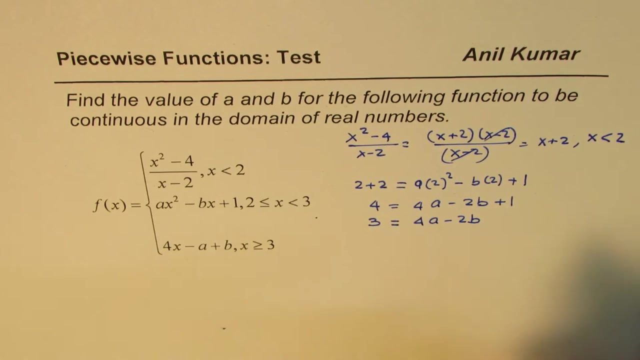 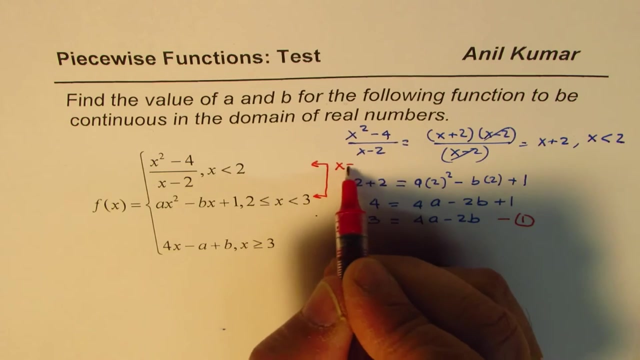 Or we say: 4 is equals to 4a minus 2b plus 1.. Taking 1 to this side, we get 3 equals to 4a minus 2b, right? So with that we get one equation. This equation we get from these two, analyzing at x, equals to 2.. Is it okay? 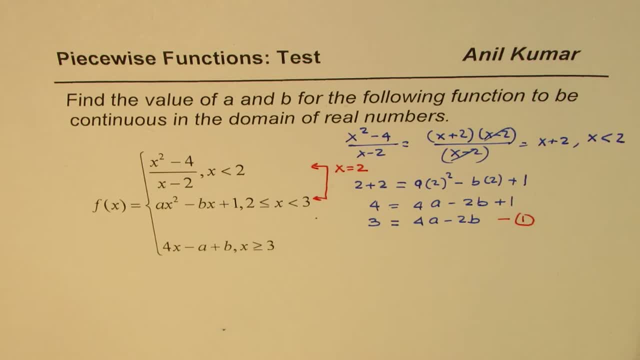 Now we can get the other equation from the other side. We can get the other two equations. We can take x equals to 3 and equate these two. So let's do that part. So when you do 3, you get a times 3 squared minus b. times 3 plus 1 should be equals to 4 times 3 minus a plus b. 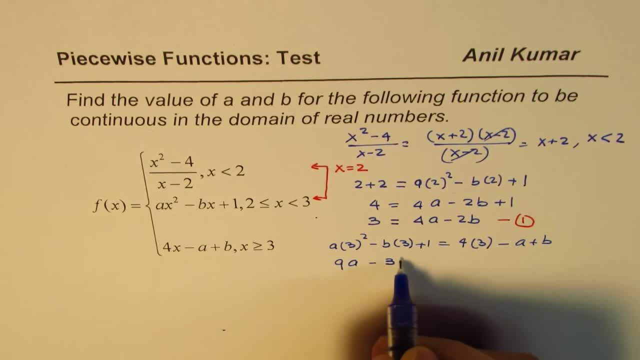 Now that gives you 9a minus 3b plus 1 equals to 12 minus a plus b. Now let's do the other part. So when you do 3, you get a times 3 squared minus b. times 3 plus 1 equals to 4 times 3 minus a plus b. 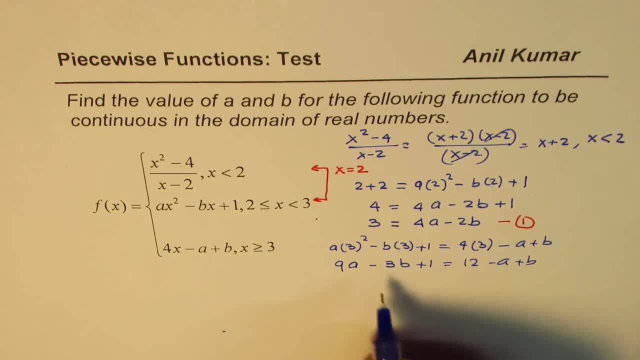 Bringing a's and b's together on the left side, this gives you 9a plus a minus 3b minus b equals to 12 minus 1, or 10a minus 4b equals to 11.. So that becomes our equation number 2.. 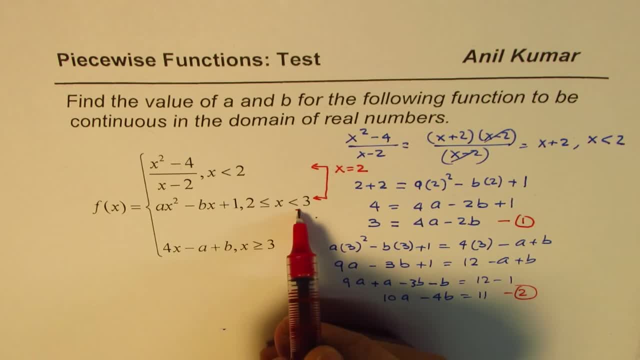 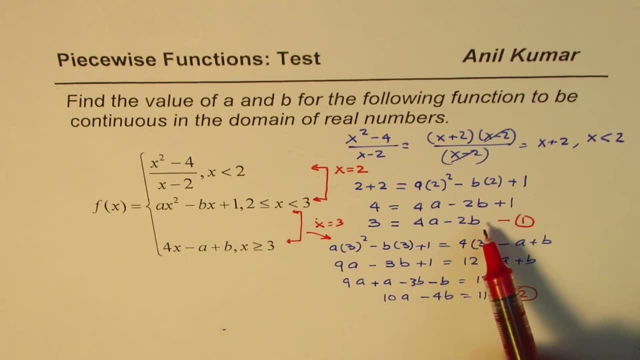 So we have two equations. So this one we got from these two for x equals to 3.. Now you could do elimination or substitution. Elimination seems to be a better option, So the equation number 1 can be multiplied by 2.. Let me do that right here, since I'm running out of space here. 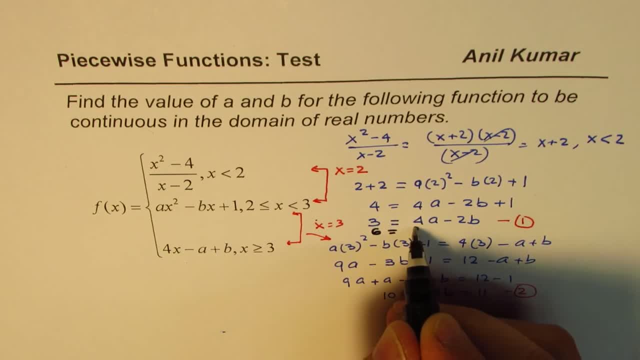 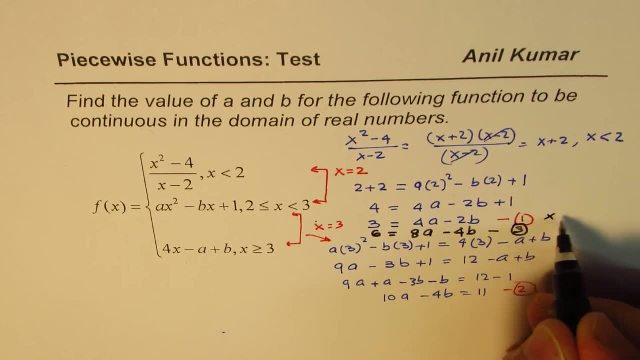 So if I times that by 2, I could write this: 6 equals to 8a minus 4b, And let me call this as my equation 3.. Is it okay? I times this one by 2.. Both sides. 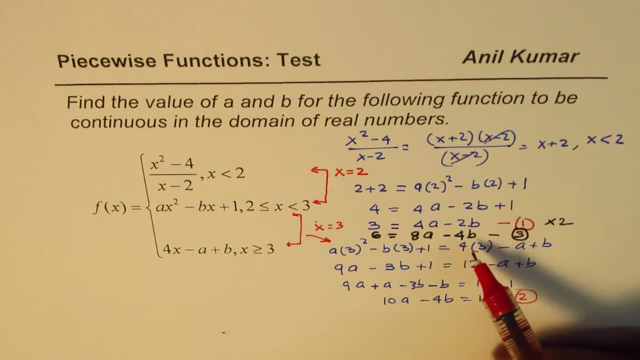 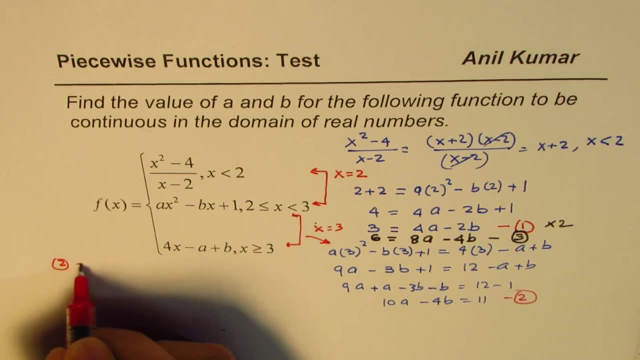 Now what we are going to do is if I subtract one from the other, that means if I do equation 2 minus 3.. So let's use this space: 2 minus 3.. Then what happens? So what we are doing now is combining. 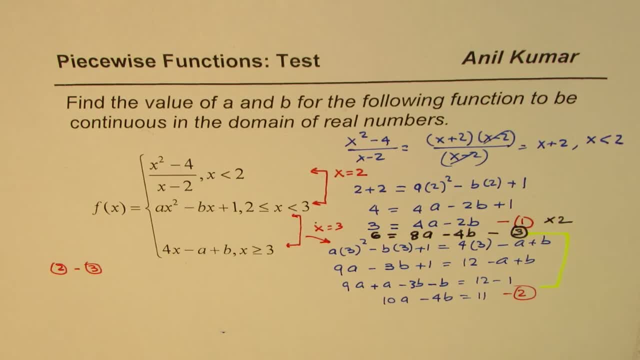 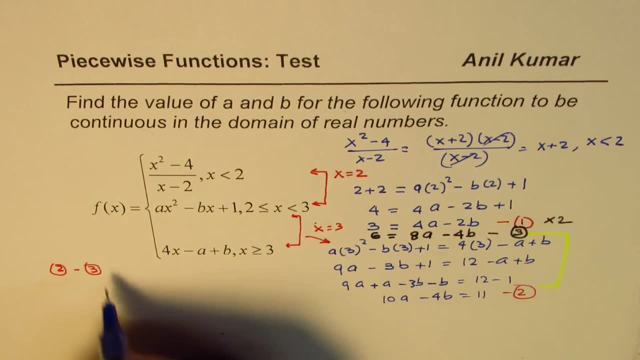 these two equations. So basically we have two equations. We have to do elimination or substitution methods to find the answer. 10a minus 8a is 2a, So we have 2a Minus 4b, minus 4b. 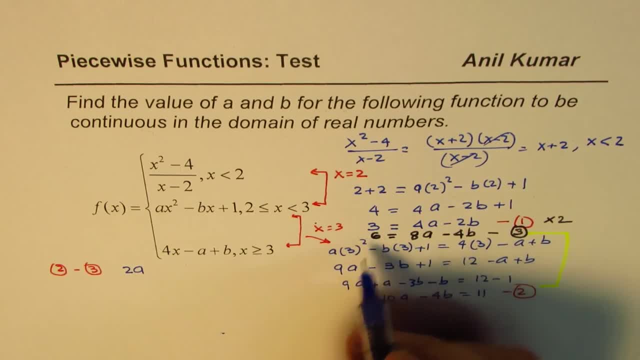 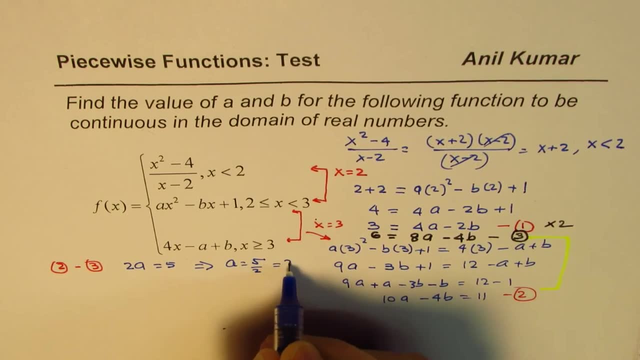 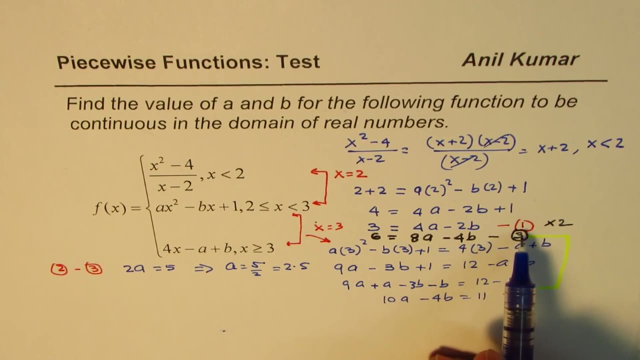 0, and here 11 minus 6 is 5, and that gives me a equals to 5 over 2 or 2.5.. Whatever, Either way. So once we have a value, we can find the value of b using one of our equations. 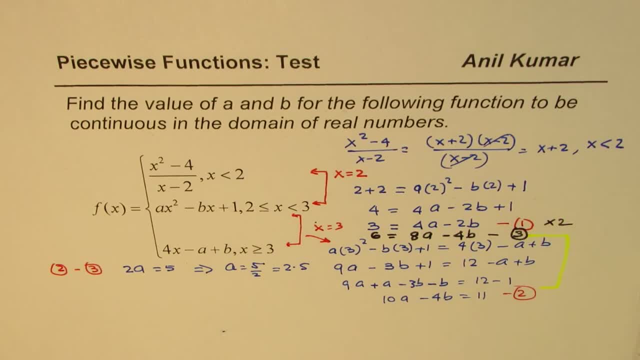 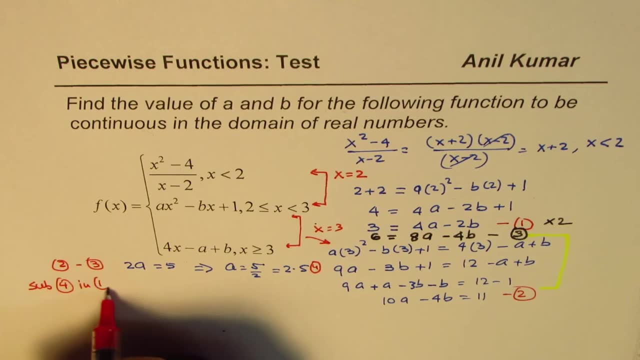 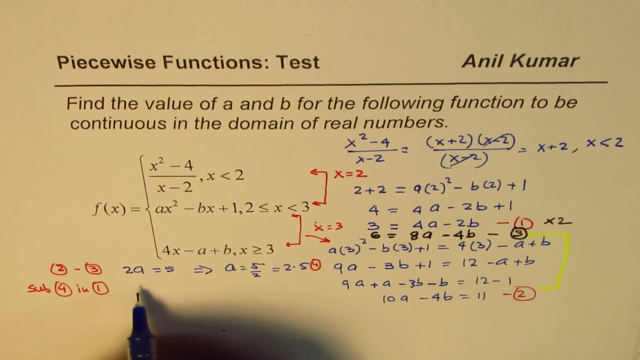 Right, So let me substitute. So now we'll call this as our equation number 4.. Is it okay? So we'll substitute 4 in 1.. These are simple steps to follow. 4 is a value. We'll substitute this value in equation 1. 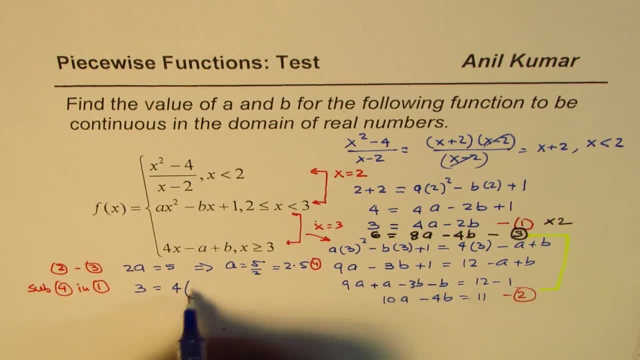 which is 3, equals to 4 times a value is 5 by 2 is better here? Okay, Minus 2b. So we get 3 equals to 5 times 20. divided by 2 is 10 minus 2b. 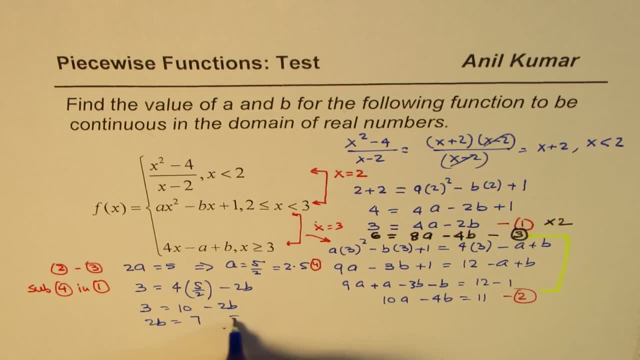 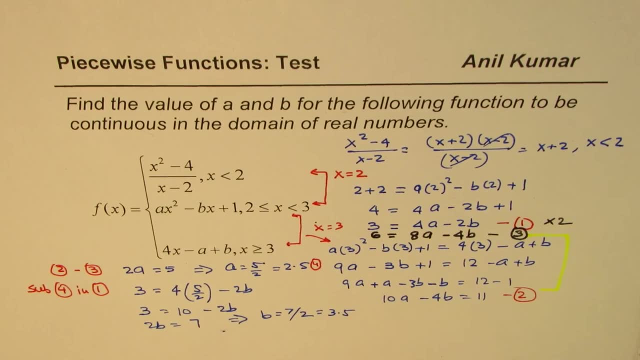 And rearranging, we get 2b equals to 7, which implies b equals to 7 over 2.. Is it okay Or 3.5. 3.5.. So we get our answer. Let me write down the answer here.